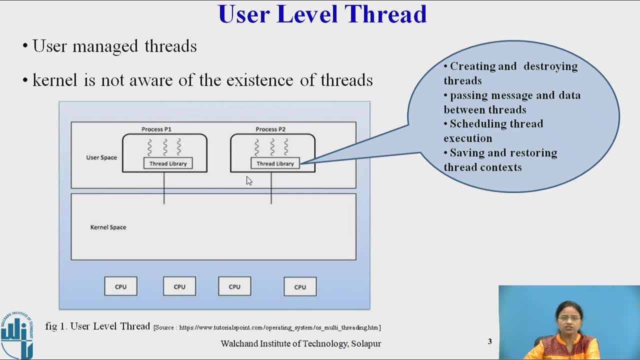 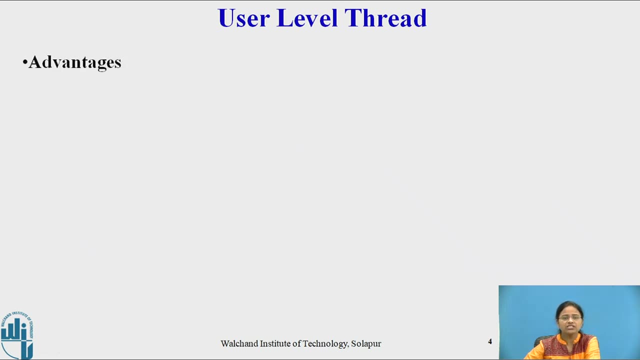 data between threads. The thread scheduling and execution is also done by thread library. Thread library also supports for saving and restoring the thread context and memory Thread whenever there is switching between the threads within a process. the advantages of user level threads are: thread switching does not require kernel mode. 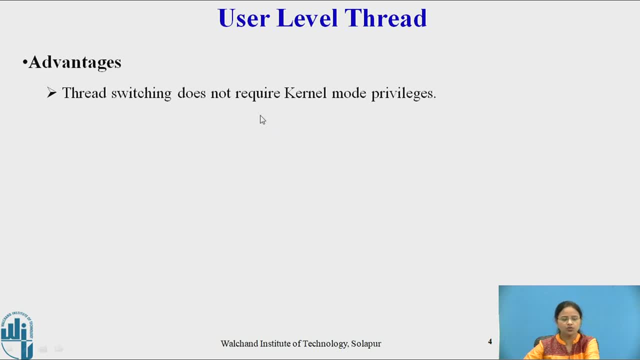 privileges because these threads are created in user space and these threads are created by user library. user level thread can run on any type of operating system. scheduling can be application specific in the user level thread. user level threads are fast to create and manage. these are all advantages of user. 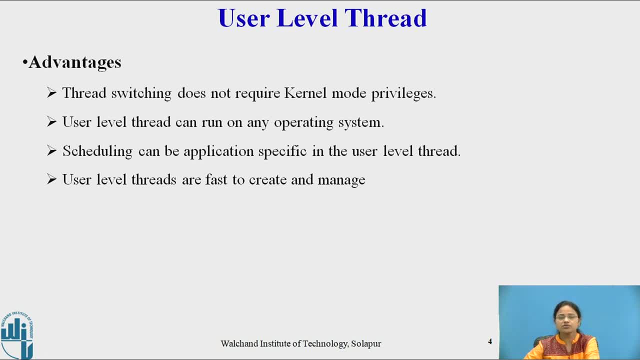 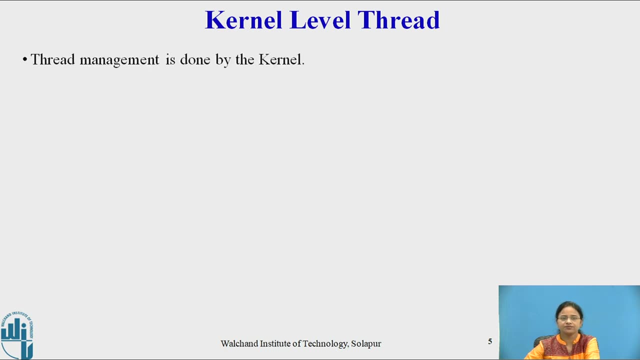 level thread only. disadvantages associated with user level thread is if use. if your system is uniprocessor system and it works on a single thread model, then if thread blocks, then whole system may block. let us see kernel level thread. here the thread management is done by kernel, no thread management code. 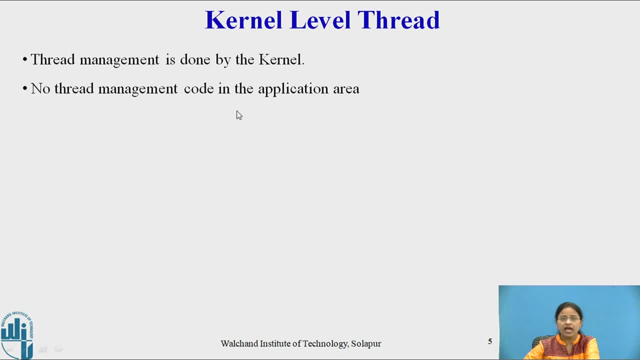 is present in application area means application area means it is user space, but it is not there. the kernel thread is not present in application area, it is only present in kernel area. so kernel threads are supported directly by operating system. any application can be programmed to be multi-threaded using kernel level. 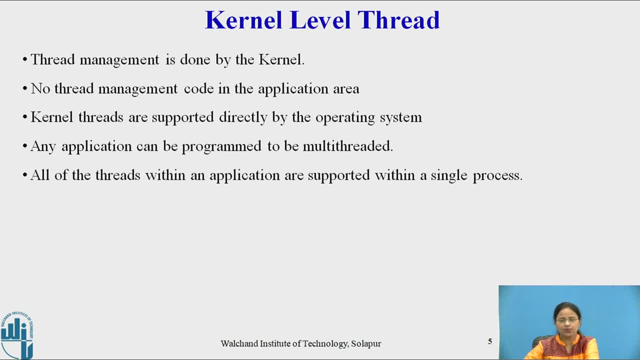 threads. all of the threads within an application are supported within a single process. kernel maintains context information for the process as a whole and for individual thread within the process. here scheduling of kernel thread is done by kernel itself and it is based on threads. the kernel performs thread creation, scheduling and 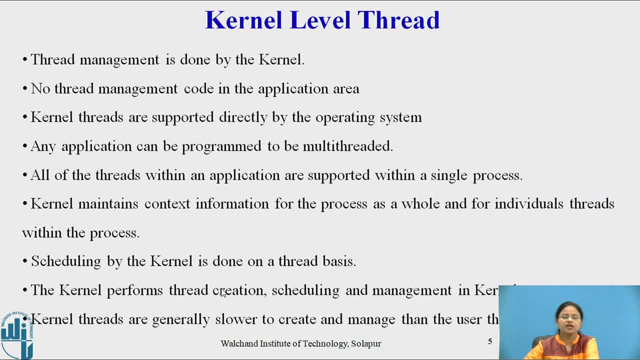 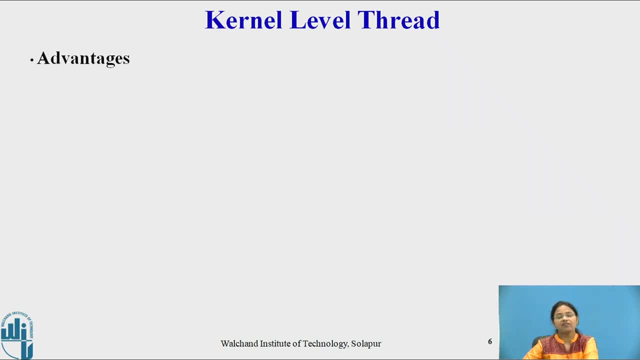 management in kernel mode. kernel threads are generally slow to create and manage than the user level threads. the advantages of kernel threads are: While kernel bits are very slow to create and manage, then users create lange. if one thread in a process is blocked, the system can add a newly created thread. 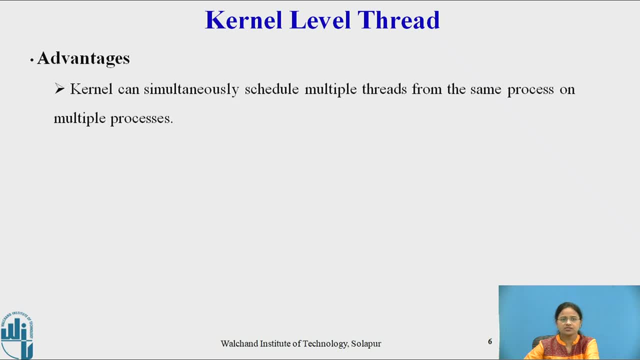 using same process. that process but system doesn't block because the requirements of the same system routines themselves can be multi. threethis advertages off kernel series tasks that we generally slow to create and manage than user level from the same process, these selbstIDs. 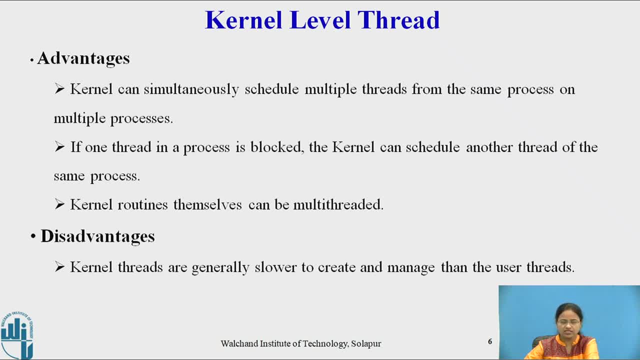 deincibur st. Uneven congressional, few like their server, individualcana DigitalNative. we know that the same principal threads- we are dying 다른 umai, because here operating system take part in creation of kernel level threads. transfer of control from one thread to another thread within the same process is user mode switch to. 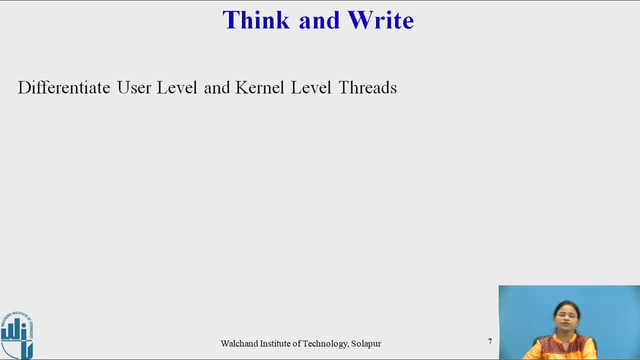 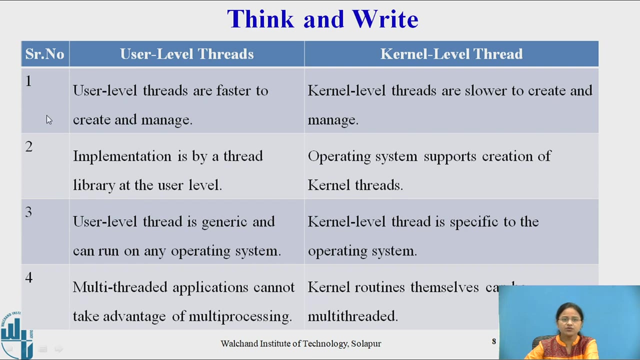 the kernel mode. now just pause a video and differentiate between user level thread and kernel level thread. okay, now let us see the difference between user level thread and kernel level thread. user level threads are faster to create and manage, while kernel level threads are slower to create and manage. the implementation is by thread library at user level, while for kernel thread operating system supports creation of kernel threads. user level thread is generic and can run on any type of operating system, While kernel level thread is specific to the operating system. Here in user level thread, multi-threaded applications cannot take advantage of multi-processing, While in kernel thread, kernel routine themselves can take an. 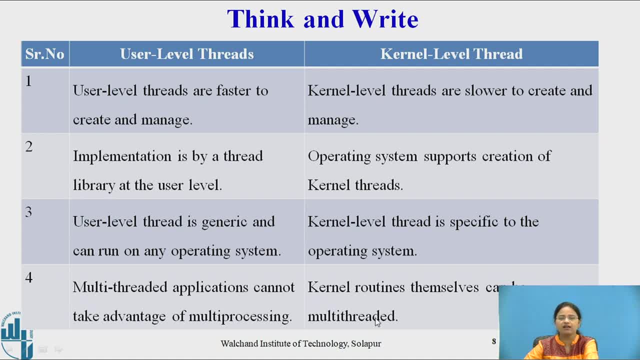 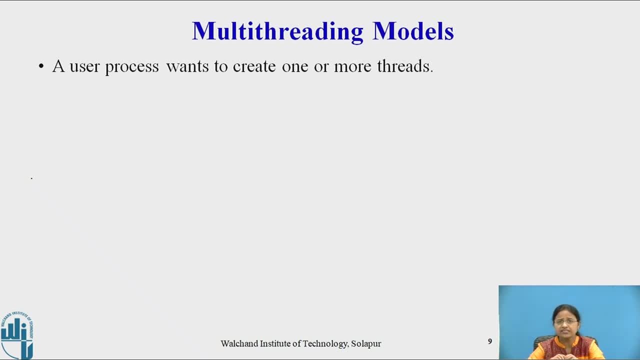 advantage of multi-threaded? because they themselves are multi-threaded. Now let us see multi-threading model. Now, what is multi-threading? Multi-threading means a process contains multiple thread which performs multiple tasks at a time. So here a user process wants to create one or more threads. 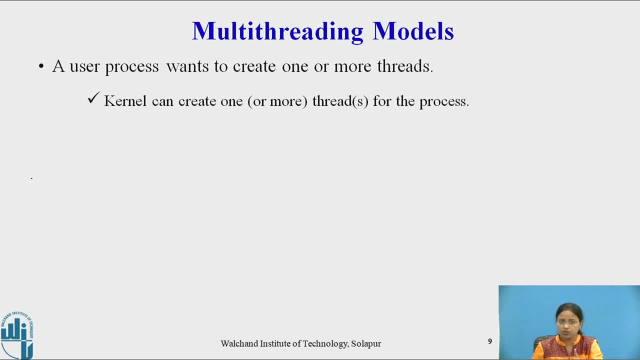 Then kernel can create one or more thread for the process. Even a kernel does not support threading. it can create one thread per process. that is, it can create a process with a single thread of control. This means that each and every process is associated with single thread of control. 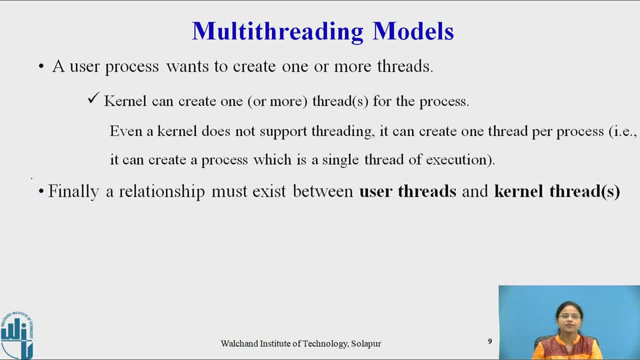 Process is associated with single thread, always. Finally, a relationship must exist between a user thread and kernel thread, because in user space also we are using process, in kernel thread also we are using process. So processes, each process is associated with thread. So there must be relationship between user thread and kernel. 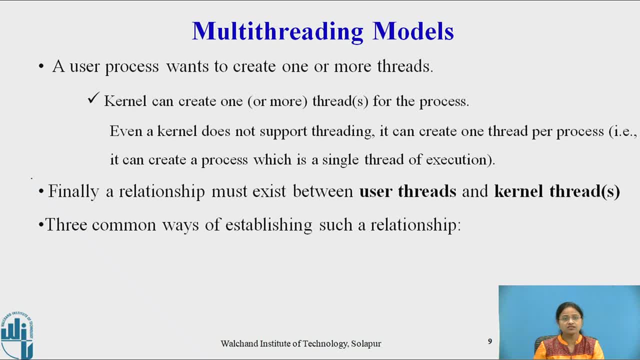 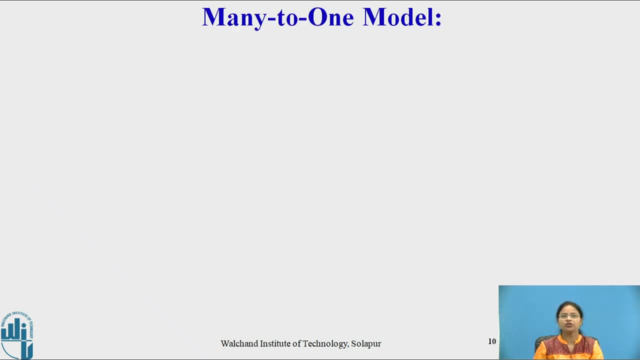 There exist three common ways of establishing such a relationship. that is, many to one model, one to one model and many to many model. Let us see these models in detail. First model is many to one model. Now in many to one model, we have many user level threads. map to single kernel level thread. 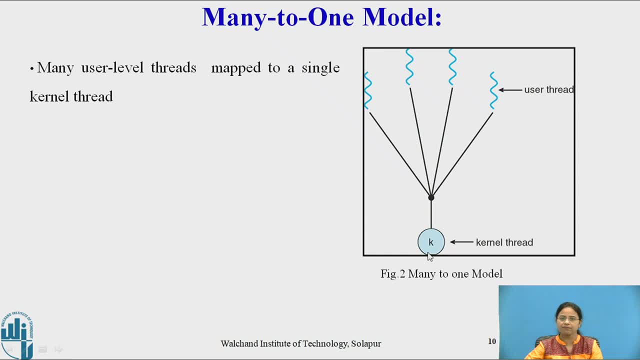 as shown in this figure, We have many user level threads which are mapped to single kernel level thread. Here these type of threads are used in solaris green threads or GNU portable threads. All these user threads are created in user space using thread library. 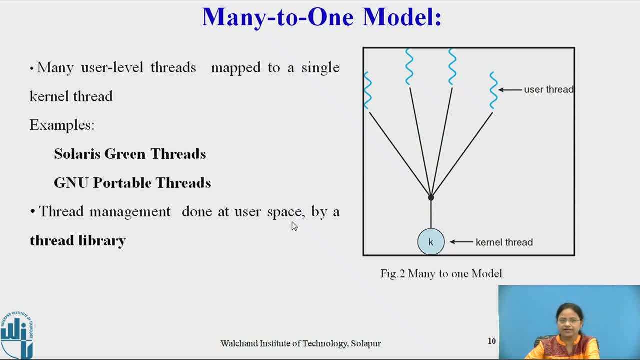 So thread management is done at user space by thread library. Kernel supports in this case kernel supports only the process concept, not the threading concepts. So only user threads are created in user mode and they are mapped to single kernel thread. Only one user thread can use a kernel thread at a time. 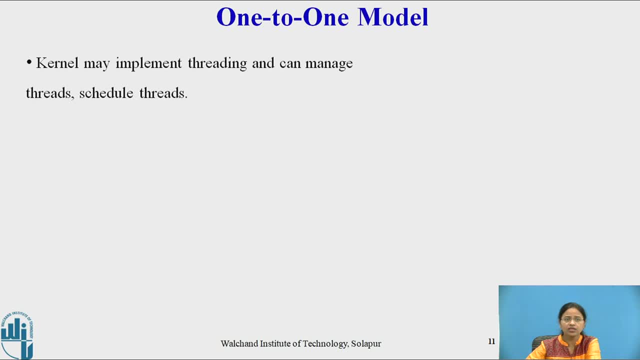 Next model is one to one model. Now here kernel may implement threading and can manage threads schedule and they can also schedule threads. Now, as shown here, one to one model: here each user level thread is mapped to single kernel thread, So each kernel level thread. so mapping is one to one, that user level thread is created. 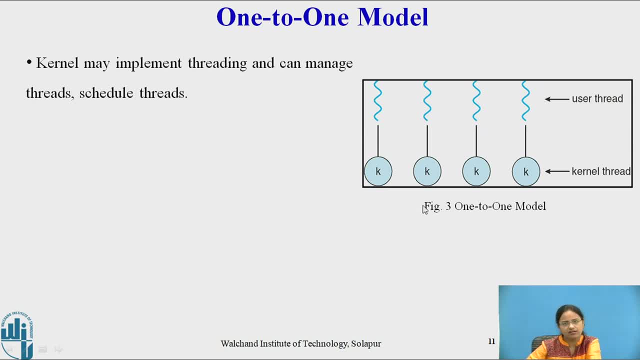 at user space using thread library and kernel level. threads are created at kernel using operating system. Now here, kernel is aware of all these threads. So recent operating systems- windows, linux, all operating systems supports this one to one model, All these kernels having thread support. 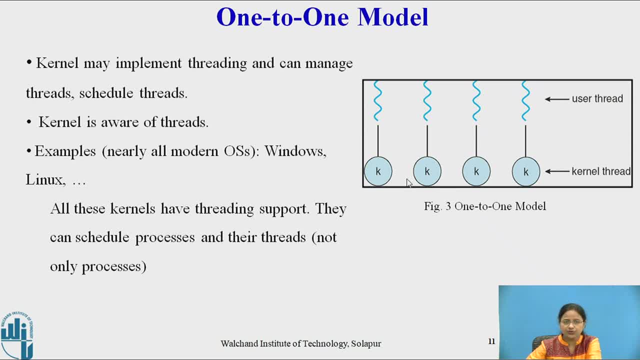 So kernel is aware of all these threads. So kernel is aware of all these threads, They can schedule processes and their threads. then not only the process means in this case: whenever kernel schedules a process, it schedules process along with its thread. not only it does not schedule only the process. 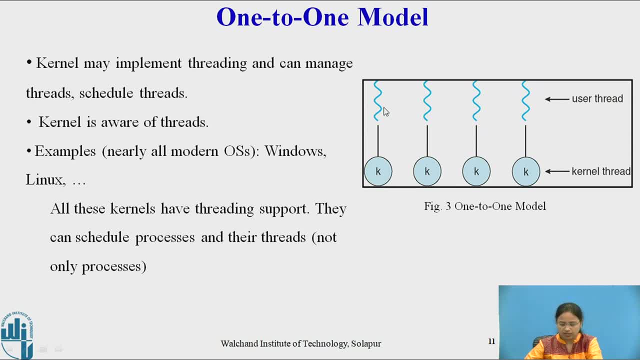 So thread scheduling is also done. So this is what the user and kernel model, that is one to one model. each user thread is mapped to each kernel level thread. This is what the kernel model can do. Now. next model is many to many model.